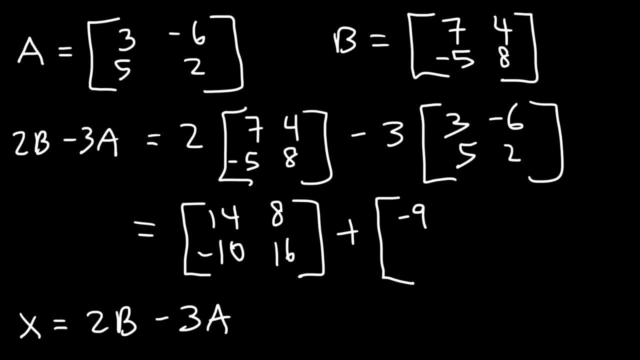 So negative 3 times 3 is negative 9, negative 3 times negative 6,, that's positive 18.. And then negative 3 times 5 is negative 15, and negative 3 times 2 is negative 6.. 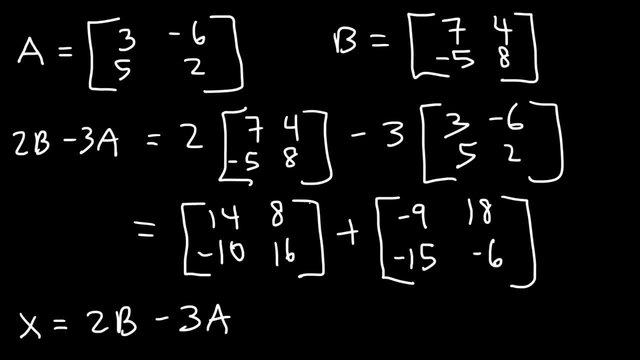 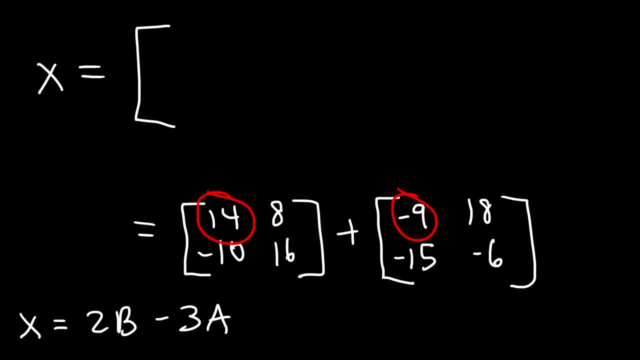 So now all I need to do is add these two matrices. So matrix X is going to have the following values: So first let's add 14.. So we have 14 and negative 9, which is the same as 14 minus 9, so that's going to be 5.. 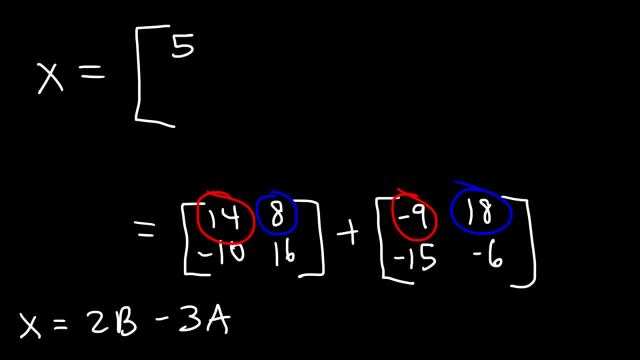 And then we have 8 plus 18,, which is 26. And then negative 10 plus negative 15,, that's negative 25.. And then 16 plus negative 6, which is 10.. And so that's the value of matrix X. 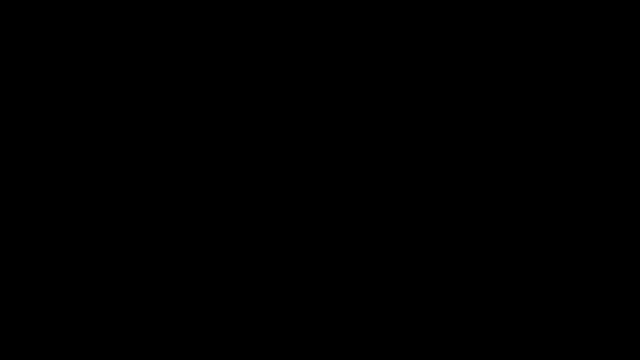 So that's how you can solve for the missing matrix. Now let's work on another example. So let's say we have matrix A. It has the numbers 2,, 7, negative 4, 5, negative 3, and 9.. 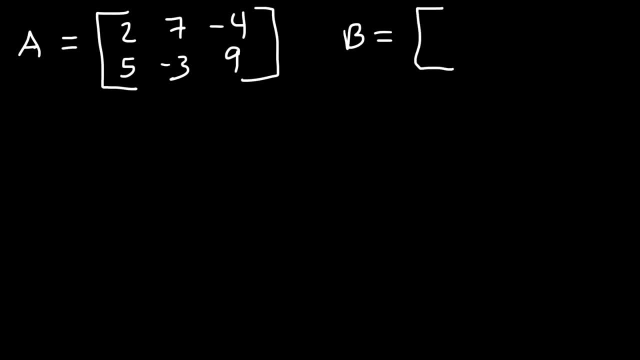 And matrix B is also going to be a 2 by 3 matrix. It's going to have two rows, three columns, So let's say it's 4, negative, 6, 5, negative, 2, 1, and 3.. 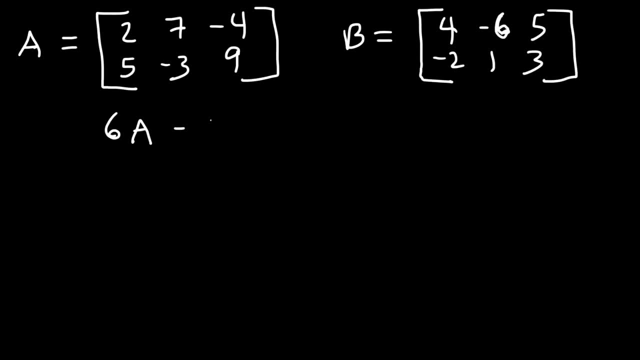 And here is the matrix A, the equation. we're going to say that 6a minus 2x is equal to 4b. so determine all of the elements in matrix x. so let's solve for x. let's subtract both sides by 6a. 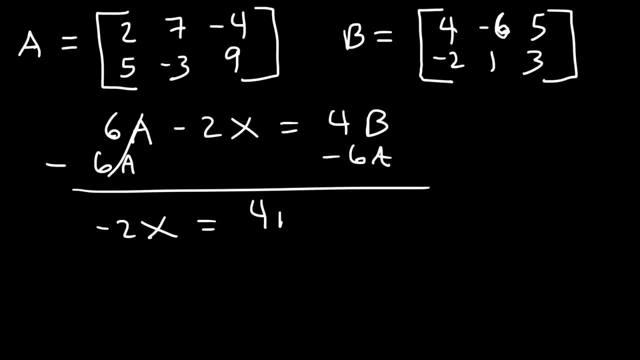 and so we can see that negative 2x is equal to 4b minus 6a. and then let's divide every term by negative 2.. so x is going to equal 4, divided by negative 2 is negative 2, negative 6. 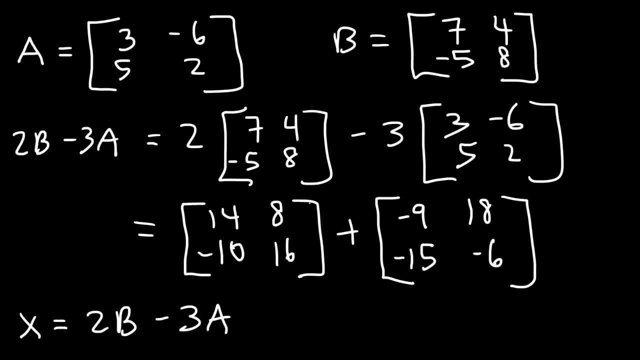 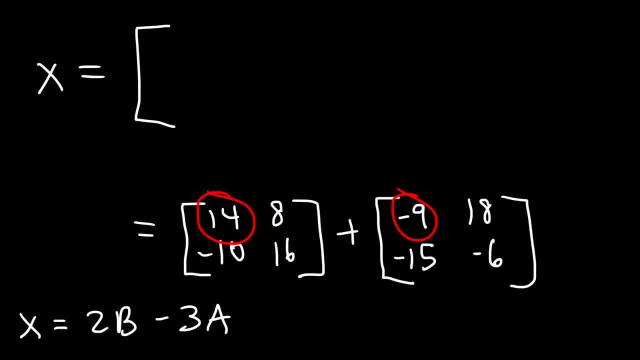 So now all I need to do is add these two matrices. So matrix X is going to have the following values. So first, let's add 14. And negative 9, which is the same as 14 minus 9, so that's going to be 5. And then we have 8 plus 18, which is 26. And then negative 10 plus negative 15, that's negative 25. And then 16 plus negative 6, which is 10. And so that's the value of matrix X. So that's how you can solve for the missing matrix. 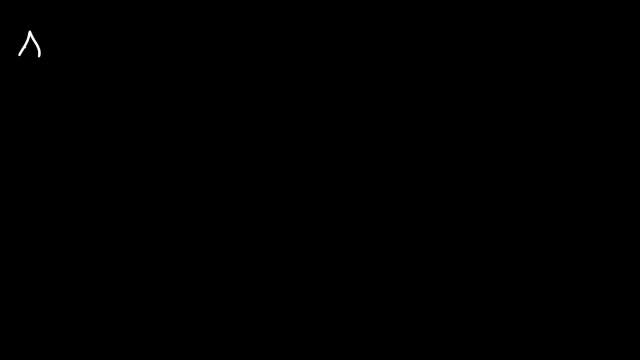 Now let's work on another example. So let's say we have matrix A. It has the numbers 2, 7, negative 4, 5, negative 3, and 9. And matrix B is also going to be a 2 by 3 matrix. It's going to have two rows, three columns. So let's say it's 4, negative 6, 5, negative 2, 1, and 3. And here is the matrix B. And here is the equation. 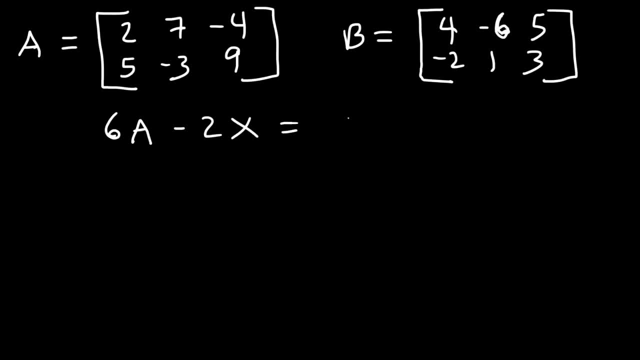 We're going to say that 6A minus 2X is equal to 4B. So determine all of the elements in matrix X. So let's solve for X. Let's subtract both sides by 6A. And so we can see that negative 2X is equal to 4B minus 6A. And then let's divide every term by negative 2. So X is going to equal 4 divided by negative 2. 4 divided by negative 2 is negative 2. Negative 6 divided by negative 2 is positive 3. 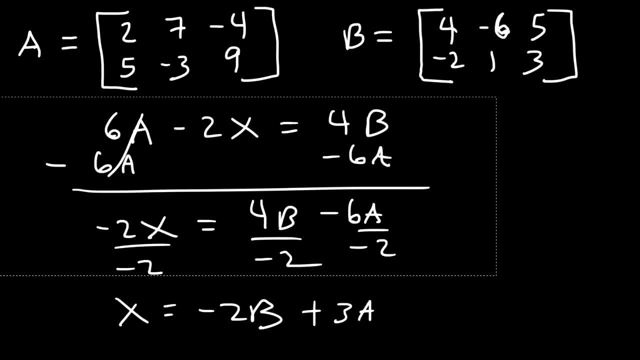 So I'm going to reverse 3A and negative 2B. So matrix X is equal to 3A minus 2B. And so that's going to be 3 times matrix A minus 2 times matrix B.